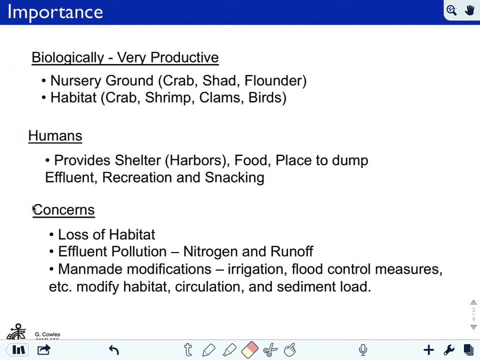 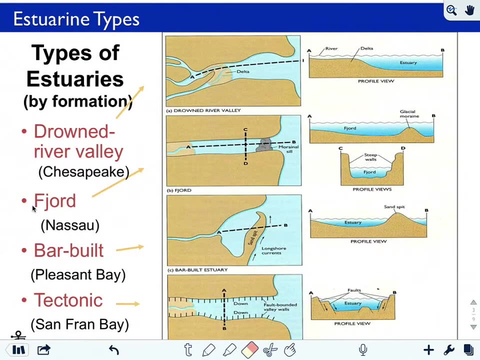 And there's a lot of concern about loss of habitat and the effluence from wastewater systems reaching these habitats and modifying the ecological productivity of them. There's four types of estuaries when we look at from the point of view of their formation, So these are very long timescales. These are geologic timescales leading to the development of these estuaries, which can persist in some places for a very long time. 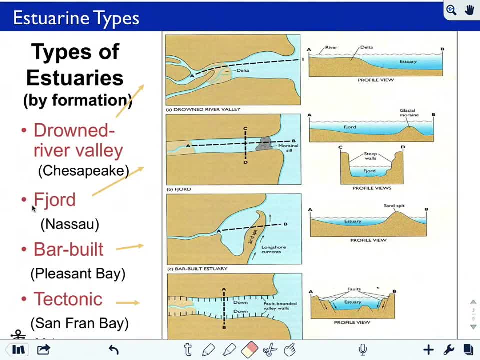 And in other places. estuaries and geological time come and go. First is the Drown River Valley. An example of that would be the Chesapeake. Essentially, during the last ice period, ice had consumed much of the waters of the world. It was tied up in ice, so the sea water sea level is about 100 meters lower than it is now. 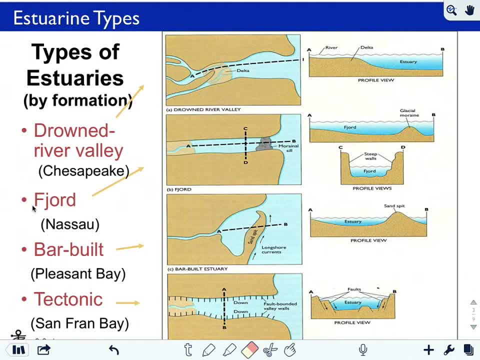 As these began to melt, they formed rivers, runoff rivers very large scale, which essentially scoured the estuaries. You can still see have a sense of the Chesapeake runoff in the canyons that run lead from the Chesapeake off the shelf. They're underwater now but at one point they were the riverbed of the Chesapeake. 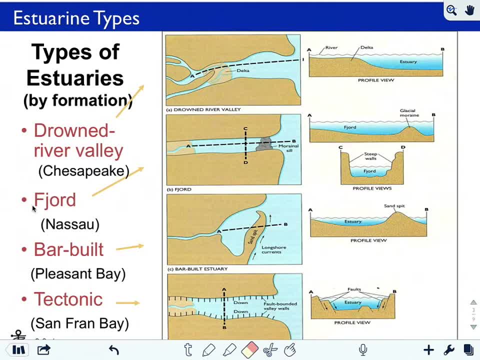 Eventually, the sea levels rose again back 100 meters up off the shelf to where we are today drowning. these old valleys, Fjord built, You can consider, glacial built. As the glaciers come out of the mountains, they push ahead of them a large amount of sediment, scouring in front of them like a bulldozer, and when they begin to recede, when they reach the edge of their 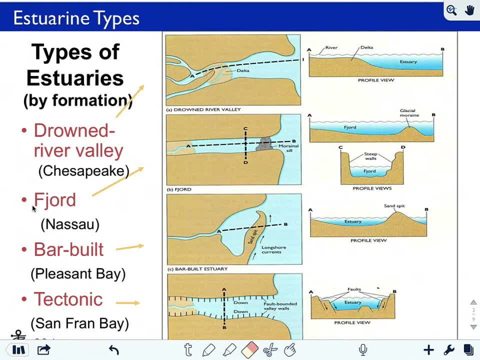 extent and recede, and they don't actually move backwards, they just they're melting faster than they're moving forward. when that leading edge recedes, it leaves behind what's called a moraine, a terminal moraine, shown in the figure here. 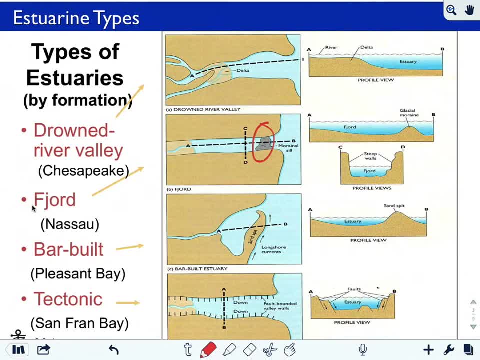 Example of a terminal moraine From the last glaciation, the Laurentide Glaciation, are the islands of Nantucket and Martha's Vineyard. Once it leaves that behind, if we look at a profile of the resulting valley, you have these fjords, and the fjords are separated from the ocean by this moraine, and often the moraine can come within a few. 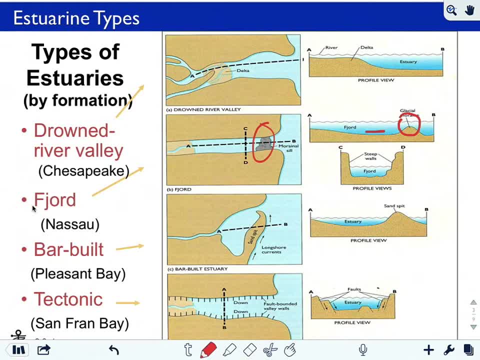 tens of meters from penetrating the surface. and what it does is it regulates the exchange of water between the fjord and the open ocean, not dissimilar from Georgia's bank being a prominent feature, but although that, it is not a terminal moraine as we understand it. 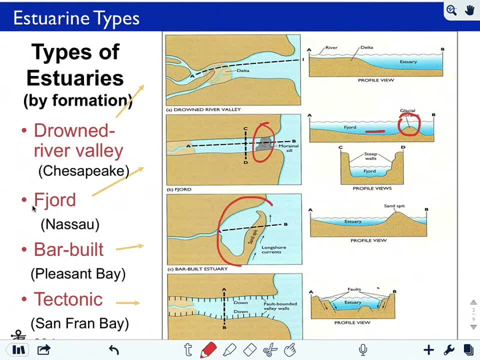 Third is a bar-built estuary. These are extremely common in our area. You have sand, spit, so you have some source of fresh water. might be a small river or an area where you have a lot of groundwater, and so there's a source of fresh water. trying to reach the bay, but along 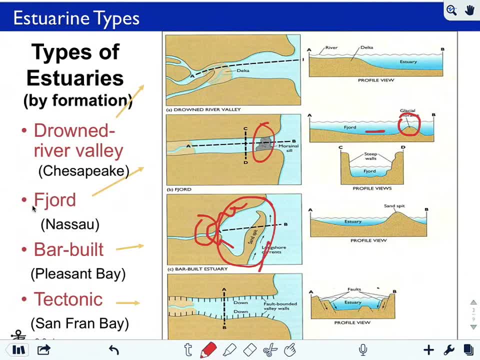 along the coast you have these longshore drift and we talked about that on the Tuesday lecture and we went over sediment transport. so essentially you have the fresh water trying to maintain the opening to this inland or harbor and the factors of sediment transport trying to close it, and sometimes one will win out of the other. you can have partial closures and then they reopen again during a storm, but these are quite common. you see spits all over, in particular Cape Cod. 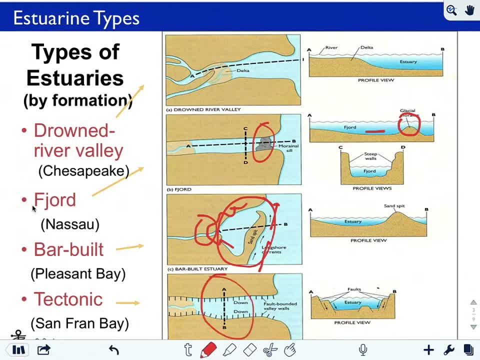 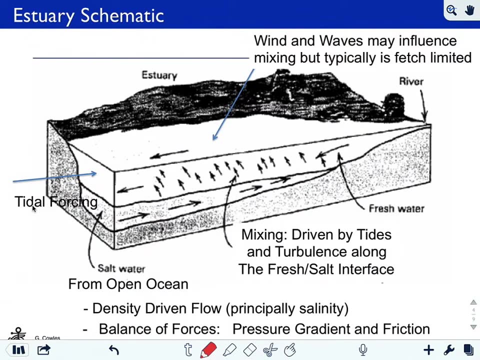 And the last is a tectonic. a great example of that is San Francisco Bay, where you have plate movement leading to the formation of an estuary or a bay. This is a general schematic of an estuary. We'll return to this point over and over again. 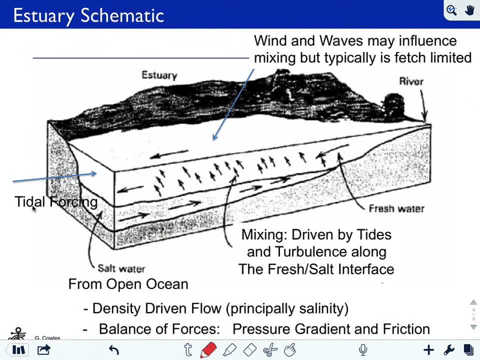 Key thing is that they're long, generally narrow compared to their length, and when I think of length, I'm thinking between where the freshwater forcing comes in at the river and the open boundary, which is where it's forced by tides from. and those are two key ingredients of an estuary: to have the tidal forcing and the riverflow. 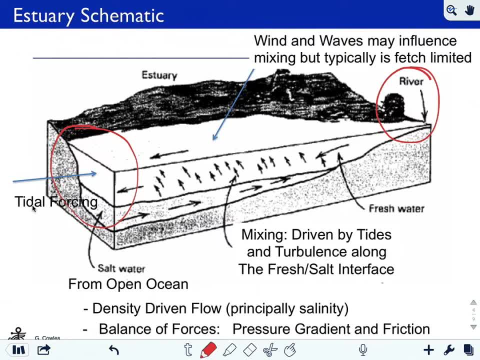 There are many places where groundwater is the primary source of the freshwater, and so those sources tend to be more diffuse along the edge of the estuary, But they tend to be long compared to their width and they are small. Both these dimensions will be small enough that rotation does not play a strong role. the earth's rotation does not play a strong role, and so these edges tend to experiment with both these idles. 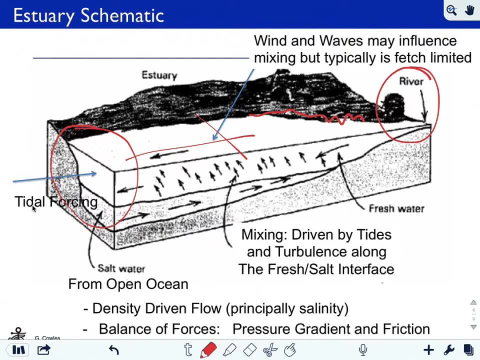 Right, and then your diffuseettuary, and so can you tell me a little bit about where that邊 goes, because then you're there and you can go further there. does not play a strong role in the dynamics of the estuary, the key driving force of fresh water. 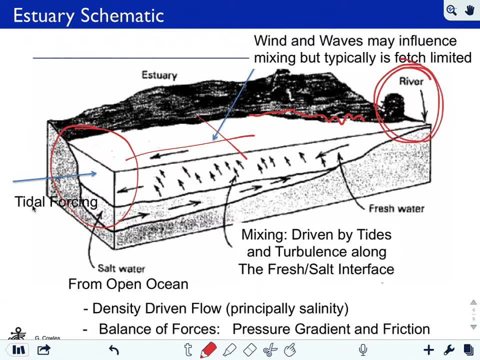 introduced by the river. so it sets up a pressure gradient which is going to force fresh water which is lighter than the seawater, so it will float on top. it will stay near the surface out towards the opening, but it doesn't move as a slab on top of the heavier water slab. there is mixing that occurs. 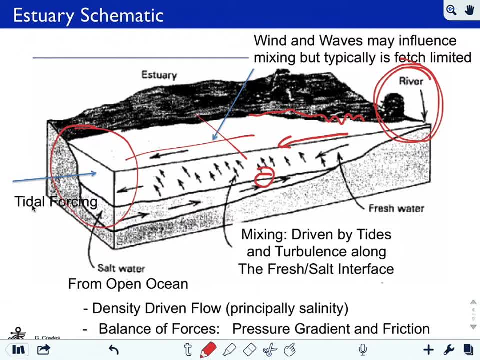 at the interface between these two fluids, and what the mixing will do is it will entrain the heavier, saltier open ocean water into this layer, creating increasing the salinity of that layer. and as the layer moves out, as this fresh water moves out, it's getting saltier and saltier as 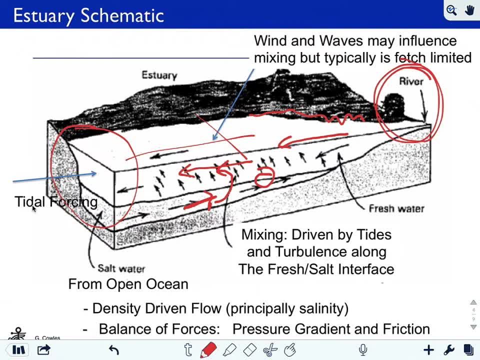 it entrains the high salinity or higher salinity open ocean water, it's entraining that volume of water as well and that. so that has to be replenished and that's replenished out here at the open boundary. so in the net you have this two-way. 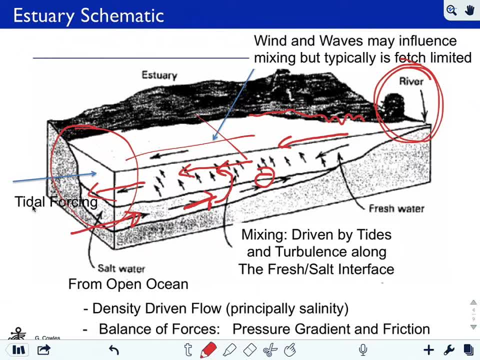 flow. now, during a course of a tidal cycle, the entire flow could be in or out, but when you average over a tidal cycle, you find out you have this two-way flow. you have inflow of higher salinity, open ocean or open bay salinity water. replacing that, the water that's been entrained. 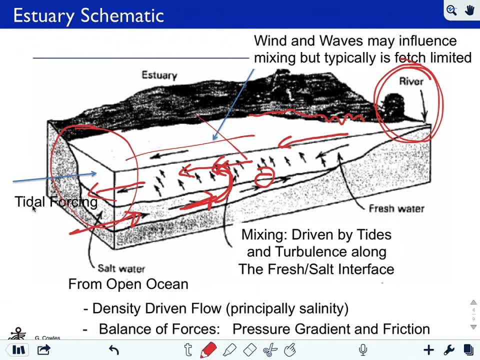 into the upper level water which is being driven by a pressure gradient by the river back out into the bay. so the two-way exchange is key because that represents a replenishment or refreshing of the water in the estuary. so the water in the estuary is not stagnant in depth, it can be quite active and it 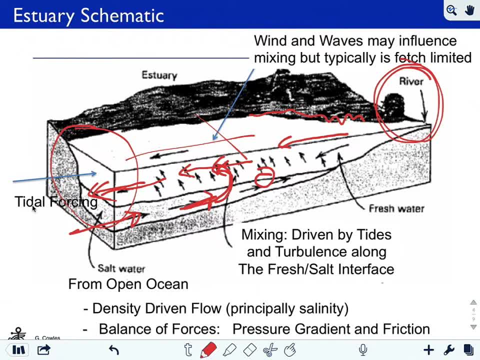 can be overturning rapidly, such that pollutants that are introduced in the estuary can be rapidly flushed out. being able to quantify the water that's being introduced into the estuary can be quite active and it can be very complicated. so quantifying that turnover time means understanding. 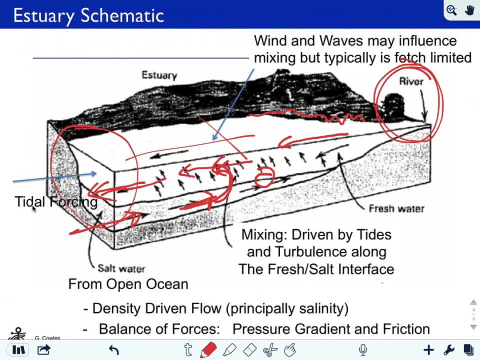 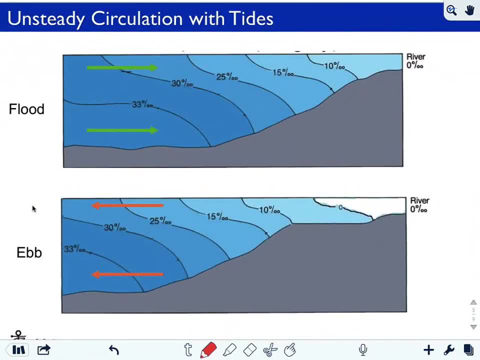 the dynamics of the estuary and being able to get at some of the key numbers that we need to make a good estimate. so with times, as i mentioned, the flow can be unidirectional, generally unidirectional. so during flood, you know, at a given station, if i put a mooring here with some adcp, so find 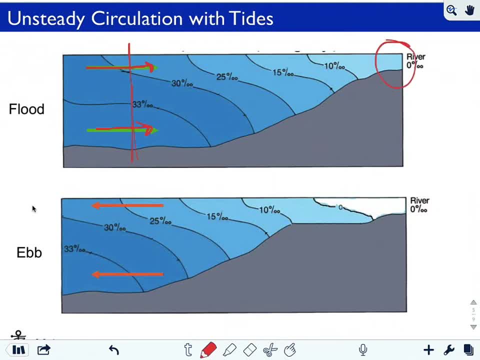 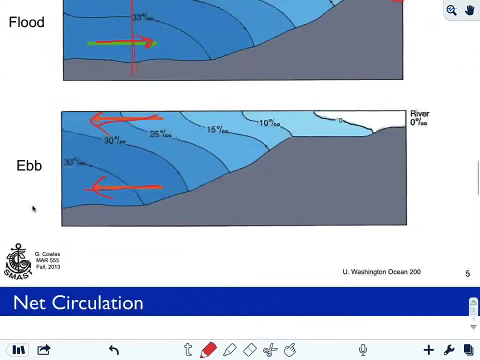 everything's moving up estuary, towards the mouth of the estuary, towards the river, or it's generally everything's moving down estuary. It's when I average over these two I find out that I have this two-way balance, that the surface, the ebb, is stronger than the flood. 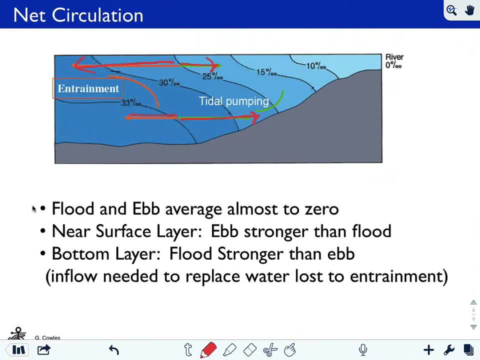 and at depth the flood is stronger than the ebb, leading to a net flow which I'll make this pink color of out at the surface and in at the bottom, when we actually average over a tidal cycle. And that's the key thing, What happens in the net over a tidal cycle And this shows you. 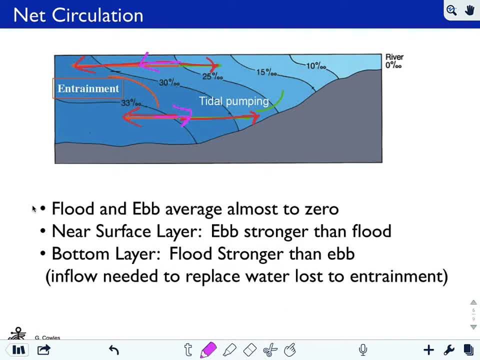 the schematic of the salinity contours You can see you have even along the surface. it starts fresh and it slowly increases in salinity as we move downstream and that's because it's entraining as it goes. it's entraining higher salinity water. You also 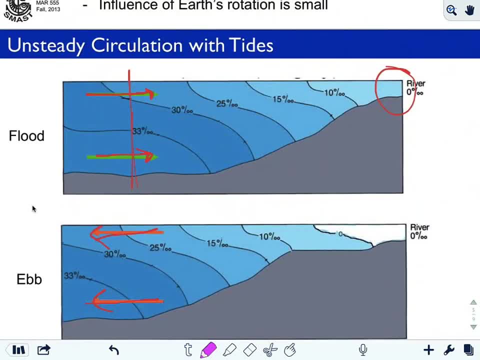 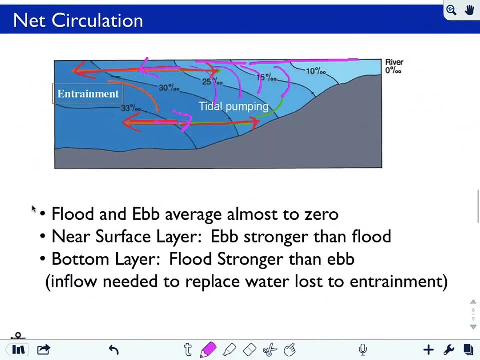 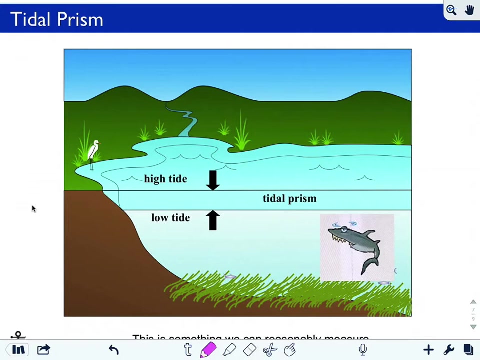 see during a tidal cycle that these isohamers, these salines, tend to get more vertical and then relax back as the water moves back and forth. So you tend to increase stratification on ebb and decrease stratification on flood. A key metric is the tidal prism and this will come up in some of the discussion we have in later. 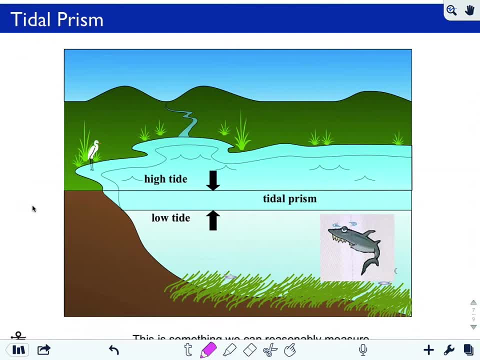 lectures as well. The tidal prism is simply the difference in the volume of water in an estuary between high tide and low tide. So high tide is more water. we subtract the water that we have at low tide and the difference between that is this tidal prism. So if you have larger tidal range, you will naturally 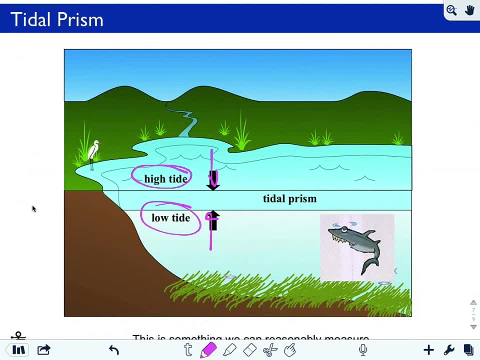 have a larger tidal prism. It's a pretty easy metric to get at because if you have some sense of the surface area of your embayment and you have some sense of the tidal range, you're essentially multiplying those two together to get a volume. So it's even with some simple 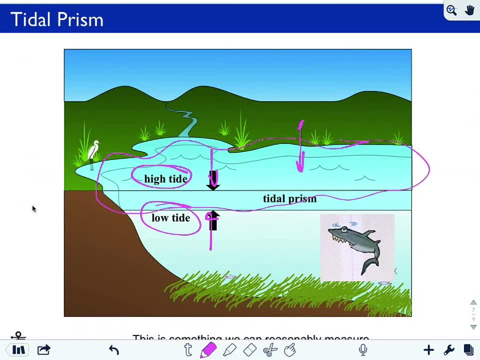 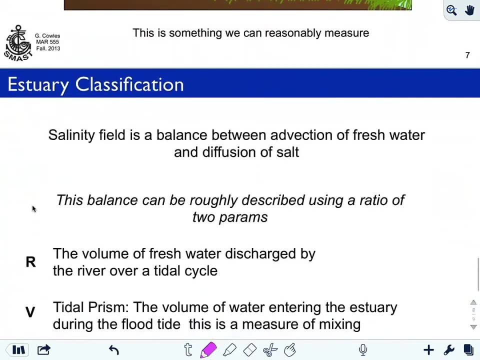 maps and some simple knowledge. it's a pretty easy metric to get at, So if you have some simple knowledge you can get a decent estimate of the tidal prism. that will be handy because that will be used in some of the estimates we come up with for. 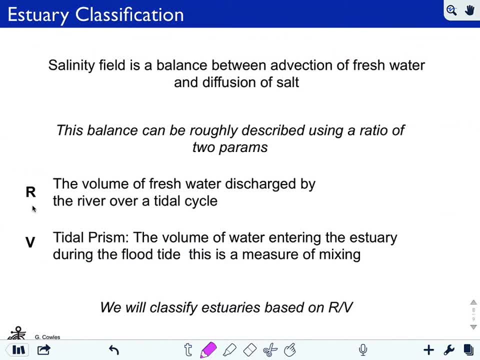 timescales. Now we can classify estuaries. A key thing that we need to consider is this balance: How much mixing is occurring? and how much mixing is occurring can be related back to two very simple things. The first is the river discharge. 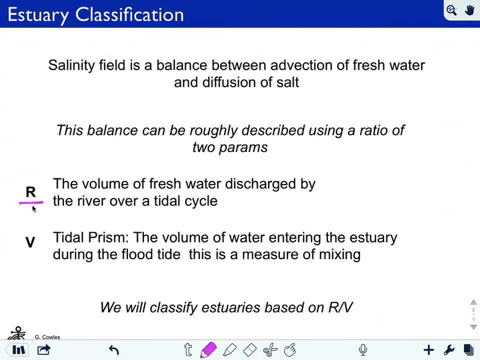 R is a volume. It's this volume of freshwater discharged by the river over a tidal cycle. So that's related to how strong tidal cycles are fixed amount of time. so how big this volume is depends on the river, the freshwater, river flux. Is it a big river? is it a small? 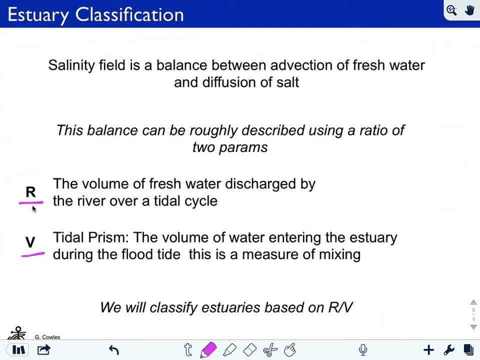 river, essentially the river discharge, And the other is this tidal prism we just talked about. R is a proxy for how much freshwater we are putting into the system. V is a proxy for how much mixing the tides are able to do, The more tides are an energy source. 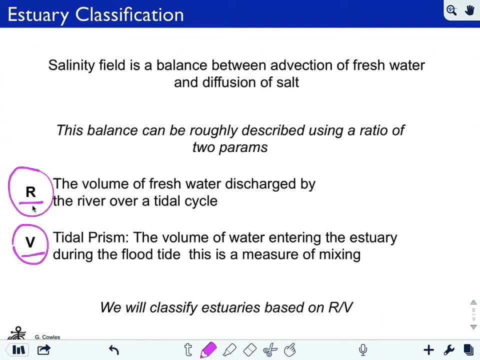 and that energy source can go into mixing. And if you have greater mixing then you have greater entrainment of the bottom water that will then need to be replenished And then you will have greater turnover and therefore a smaller timescale of flushing to the estuary. 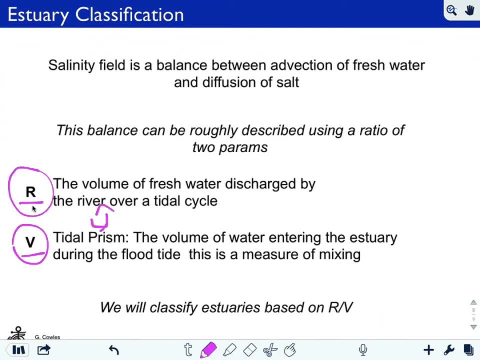 So these two things are basically fighting each other. Greater volume of freshwater discharge means that you have a lot, a lot more freshwater, and that freshwater is going to inhibit mixing because, due to maintaining the stratification, whereas the tidal prism will accentuate the mixing. So we're going to look at some classifying, some estuaries. 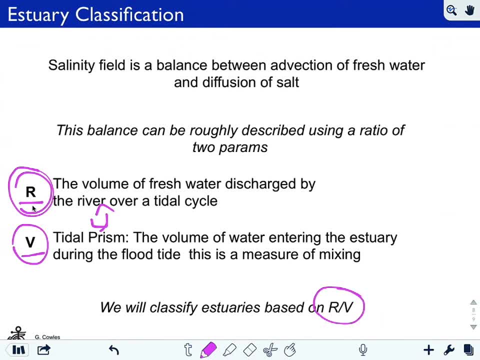 simply based on the ratio of these two quantities, both of which are fairly easy to estimate. But keep in mind when we classify these that both of these change can change with time, Particularly the freshwater. it can have a distinct seasonal cycle In our region. 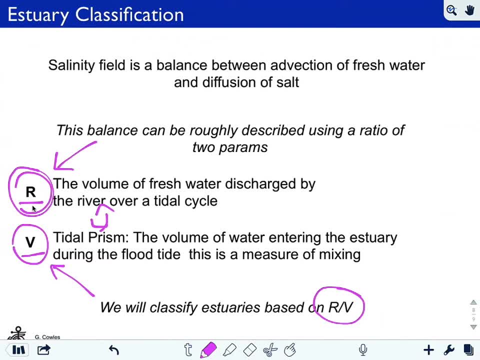 our monthly rainfalls are actually fairly similar. In some places like the Pacific Northwest, you can have two. you can have runoff of snow in the spring. so May, June, you get a big pulse and you also have a big pulse in the fall related to climate activity, storm activity. 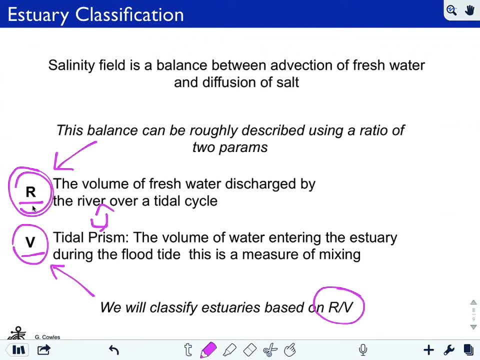 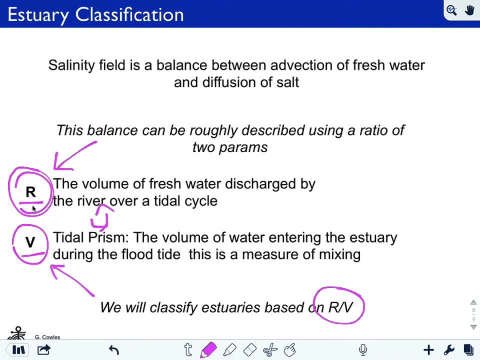 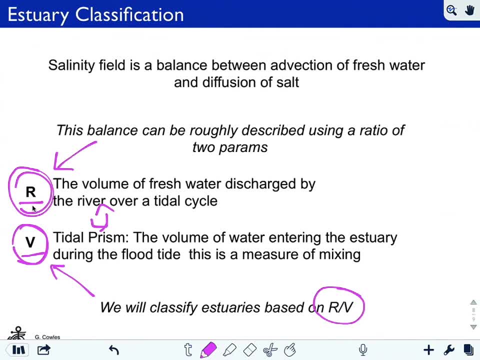 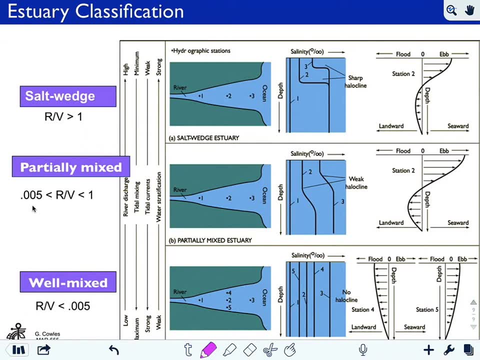 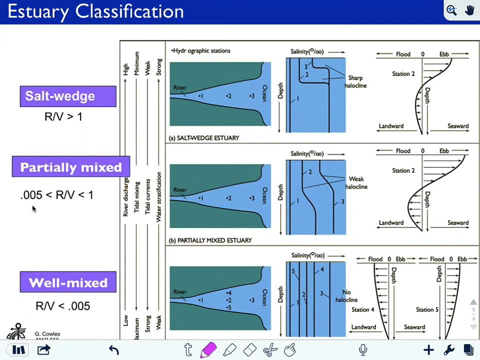 over a tidal cycle and V is the tidal prism. First is a salt wedge. A salt wedge estuary has strong river forcing compared to the tidal prism, So R over V is greater than 1.. This shows an upper view, a plan view, of the estuary. Here's the river, station 1,, station 2,. 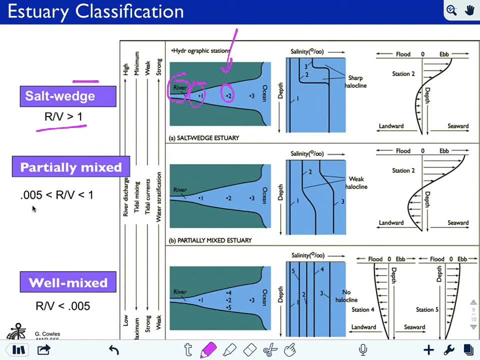 and station 3 is closest to the ocean. If we look at the profiles of salinity we see: closest to the river we have strong mixing. So right up near the river the mixing is strong enough, the tides are weak enough that essentially you have fresh water from top to bottom. 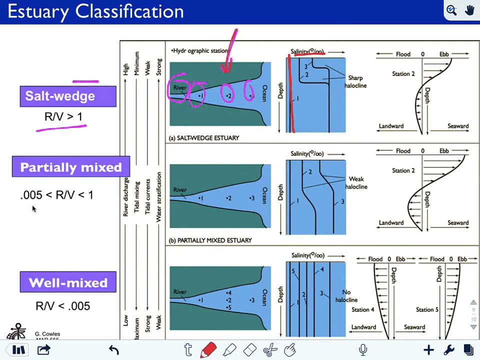 At station 2, which is the mid-estuary station. you have a sharp halo climb here. You have fresh water overlying saltier water and as it goes downstream. so weak mixing will mean that we have this halo climb, will move up and we will have. we can visualize this in a few slides. 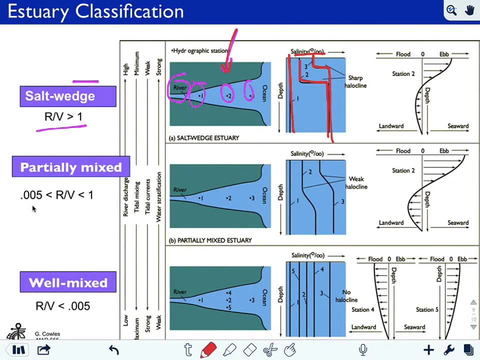 as a wedge, Essentially the pressure gradient of the river. forcing is balancing this wedge of separating the high salinity and low salinity waters, but they may remain quite separate. So you have a sharp halo climb, Which means strong stratification, which means an inhibition of the mixing. The tides are not. 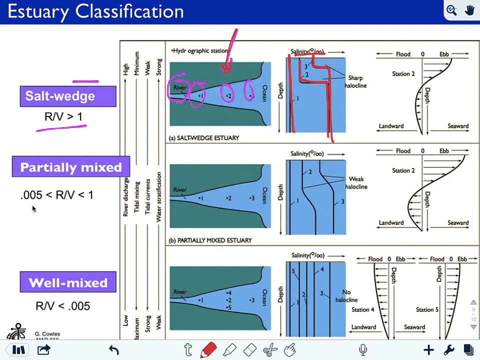 strong enough to mix down this halo climb and therefore the entrainment of the deep water is rather weak, meaning that the return flow is also rather weak because there's nothing to replenish. When we look at the net velocity profile, it looks something like this: So this is averaged. 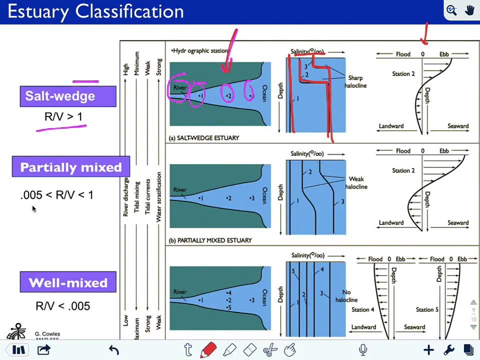 over a tidal cycle. The ebb direction is to the right and the flood direction is to the left. So at the surface you have outflow and somewhere in mid-depth is a crossover point and below that you have some inflow, but it's rather weak inflow Again, if we integrate this velocity. 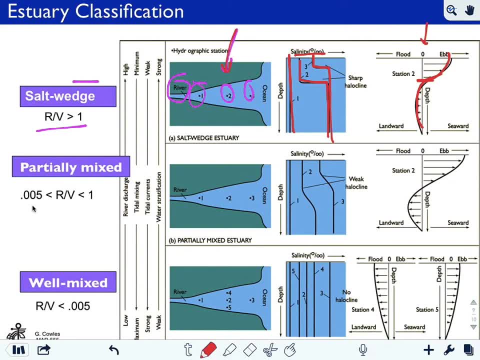 profile. we'll have a net velocity profile because the net in the net, the estuary has an outflow, It must equal the river discharge, Otherwise it will be filling up with time. So we're assuming the estuary is not filling up with time. So we have weak inflow associated with the 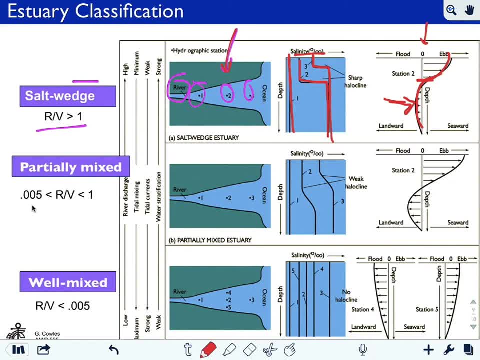 weak mixing associated with the strong river discharge, leading to large stratification. The second estuary: we've weakened the river discharge relative to the tidal prism, So now we have stronger mixing. That stronger mixing is going to weaken the halo climb. You can see a 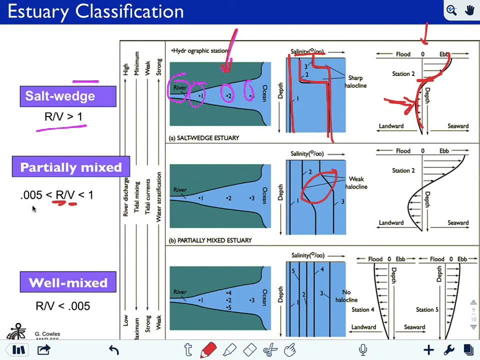 weaker halo climb here, meaning there's more entrainment, and more entrainment means more deep water that needs to come in to replenish that deep water that's been entrained into the surface layer. You can see that the return flow, the up estuary flow at depth, is stronger than it is in the salt wedge case. The net is still. 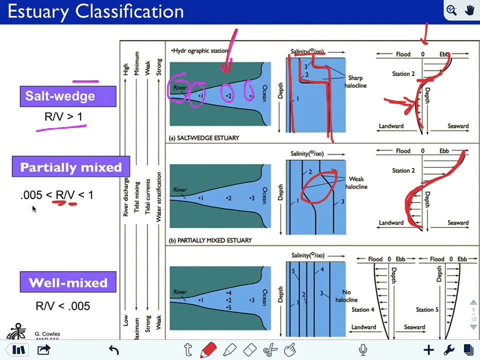 the same, so you have an enhanced outflow as well. Stronger outflow, stronger inflow. The last one example is where you have very weak river discharge compared to the volume of the tidal prism. This is probably closer to most of the estuaries in our region where the tidal forcing is strong. 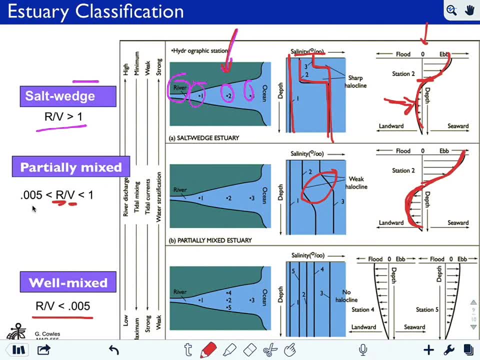 compared to the river discharge. In this case, the estuary is quite well mixed. You see very little stratification from top to bottom. You do not see any two-way flow, because we're not entraining a deeper layer. There is no deeper layer, It's simply mixed from top to 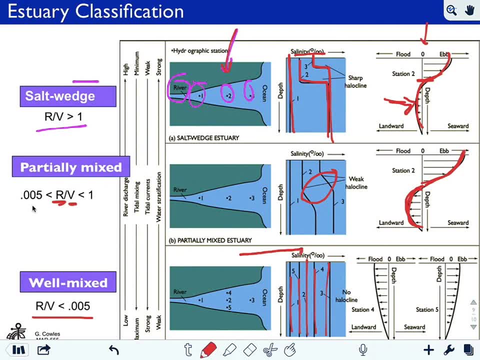 bottom. All you have is a gradient in salinity from zero at the head to open ocean, S0, at the end. And you can see that if you do profiles they're all vertical. But as you move downstream from profile one to two to three, you only see a minor variation and you only see minor.